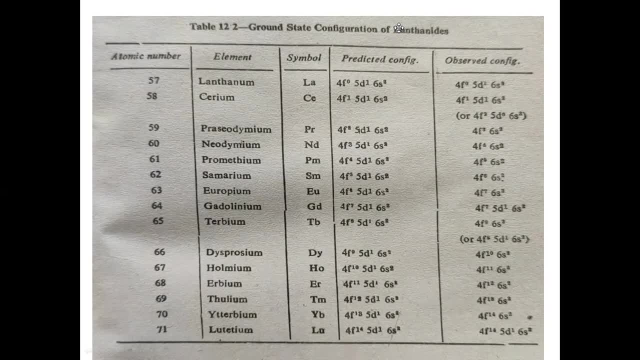 in the exams, near or far we should go for the preparation. We must prepare for that. We should not be exam-oriented. One should be knowledge-oriented. yes, what is the important source of lanthanides? lanthanide, yes, anyone monazite? okay, very good, who is going to answer? yes, your name, please. 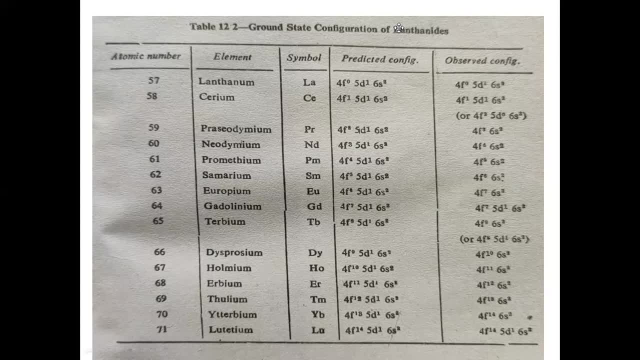 chef munaza. okay, very good. monazite sand is the important source of lanthanide. okay, it is a orthophosphate. orthophosphate is that is a mixture of lanthanide orthophosphate that is called as a what do you call monazite sand, along with lanthanide, some actinides. they are also obtained. 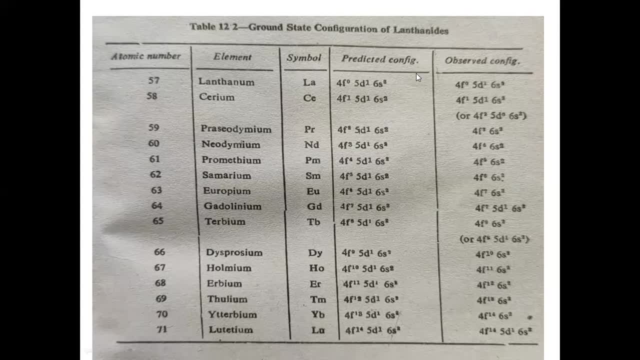 from that lanthanide from this monazite sand. but important source for lanthanide is monazite sand. so separation of lanthanides from each other or monazite sand is a difficult job, and then that can be achieved with the help of various process. we apply for that one of 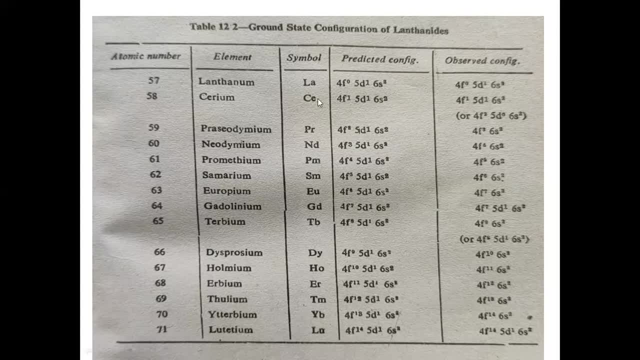 the important number of methods. are there this fractional crystallization is there? then solvent extraction is there? solvent can be extracted. fractional crystallization can be extracted. fractional crystallization is there? what is fractional crystallization? like these two things, right? suppose there is a mixture of salt. there are two salt in it. 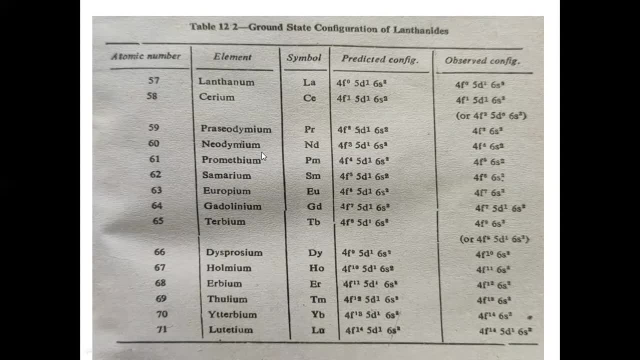 one a and b. we see in it that one of the solubility is more and the others less correct. so this principle is there in the mind. keeping into this into mind, the first crystallization will crystallize out first and the second one will crystallize out later. 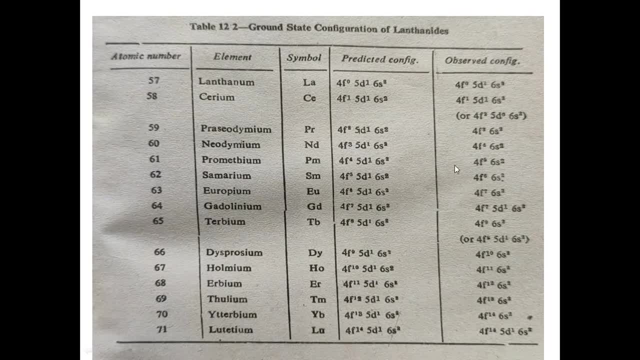 this is the principle of fractional crystallization. this is the principle of fractional crystallization. the first crystallization will crystallize out later. we will keep it in the mixture and we will cool it. we will cool it, and the first crystallization will crystallize out later. 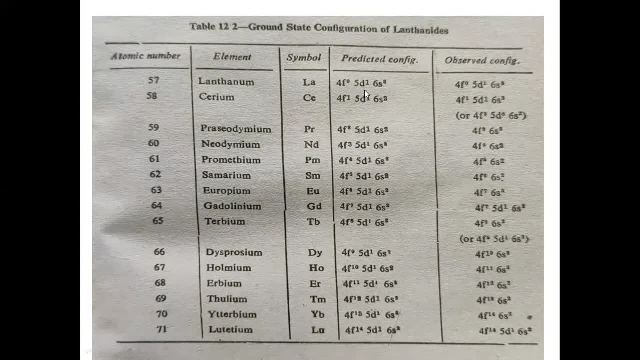 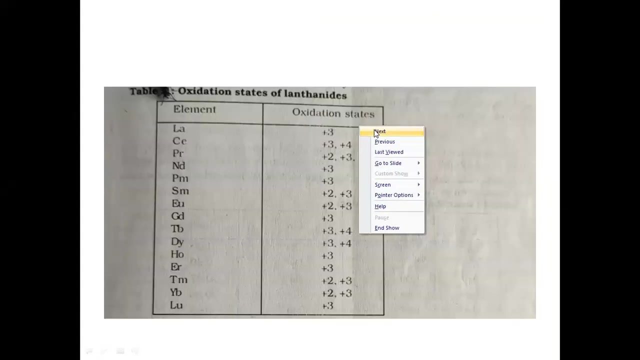 ok, we will separate it. we will filter it and separate it. whatever is left will be second, then we can heat it. this is how fractional crystallization is there. second method is solvent extraction and the third effective method is ion exchange method. very effective method: ion exchange method. 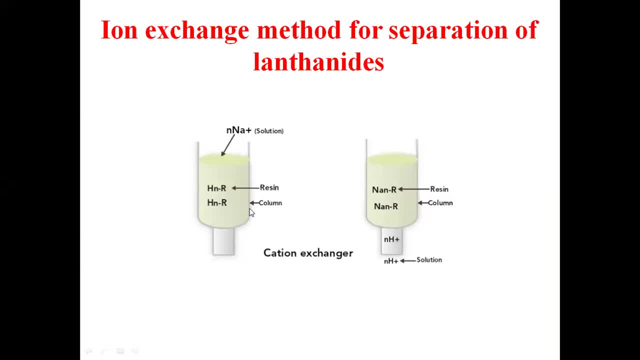 what happens in ion exchange method. this is how a burette is formed. so type of burette is there? that burette is packed with the column which is containing resin. resin means these are the fine particles, just like mustard. what is mustard? what is mustard? what is mustard? 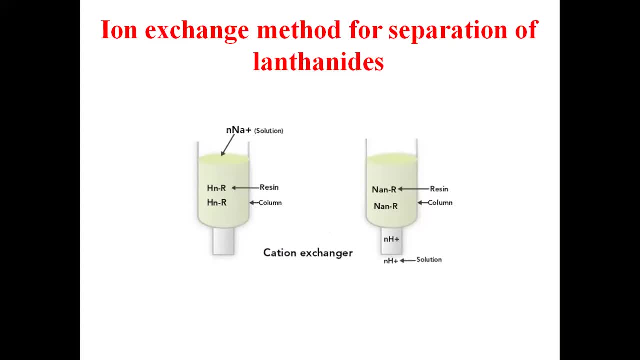 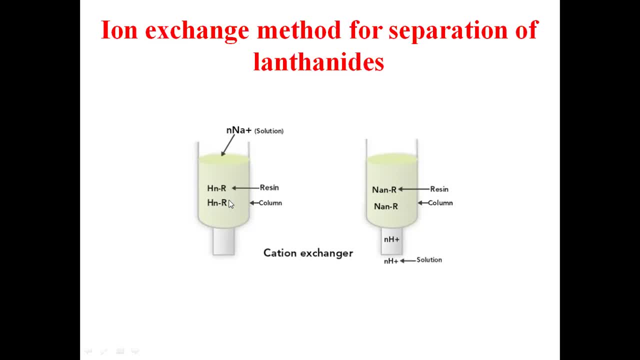 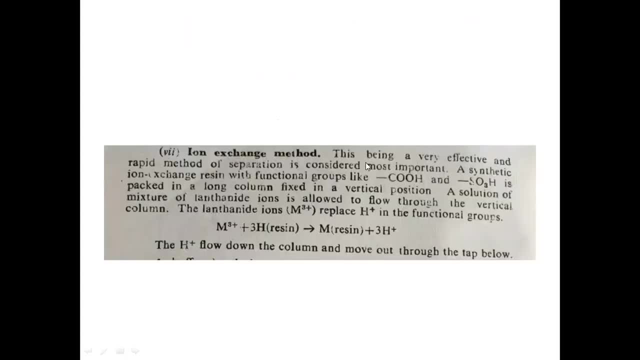 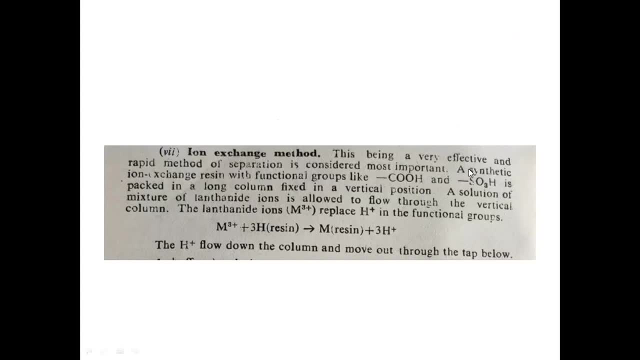 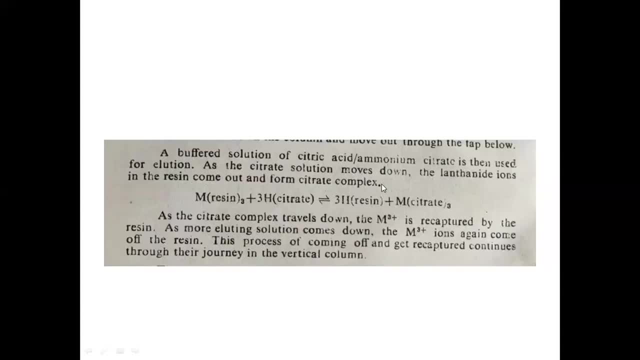 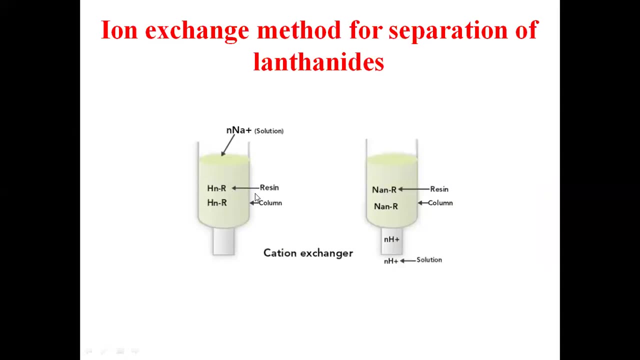 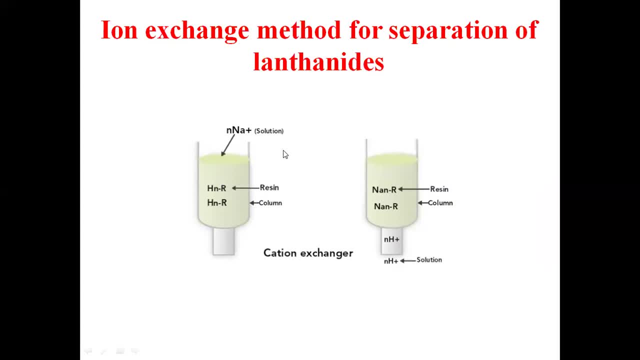 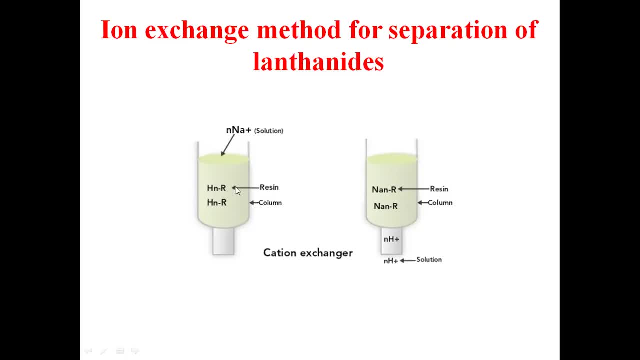 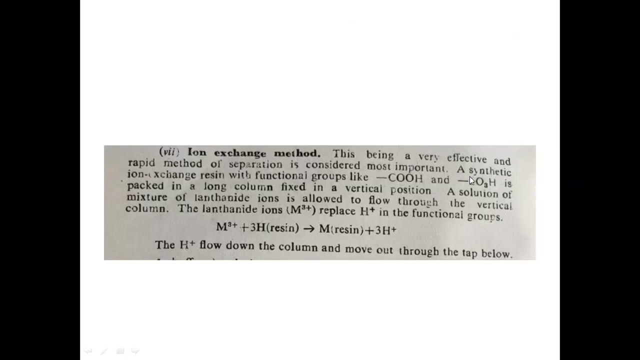 man-made. this resin contains mainly two types of two types of functional group. one is coh group, another is sulfonic acid group, so3 age group. okay, so a synthetic resin is there which has functional groups like coh and so3h group. a solution of mixture of lanthanide is allowed to flow through this column, okay. 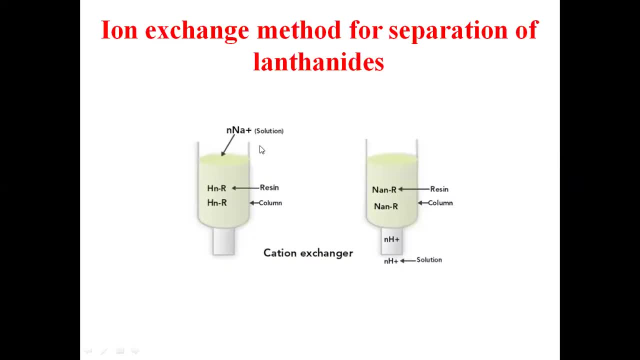 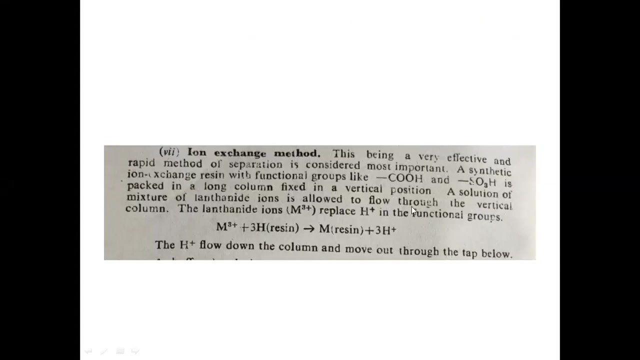 a mixture of lanthanide is powered, a solution of mixture of length and height is allowed to flow through this column. what happens? the length and height ion, m3 plus characteristic oxidation state of this length and height ion is 3 plus. so what does they do this length and height ion replace the 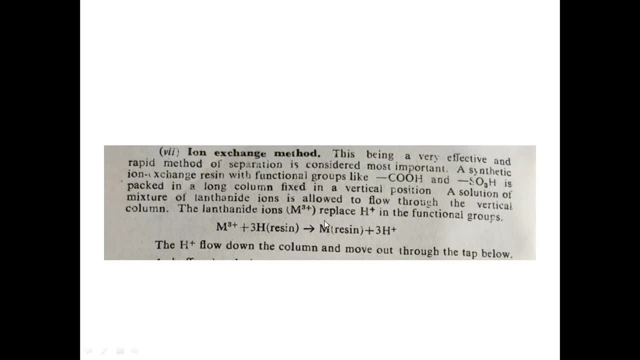 h plus ion from the functional groups. which functional group are present in the resin? yes, yes, resin, make a step to functional group coh 3h. yes, here is a hydrogen atom, here is a hydrogen atom. so what they do, what they do? what they do is they replace the length and height ion. 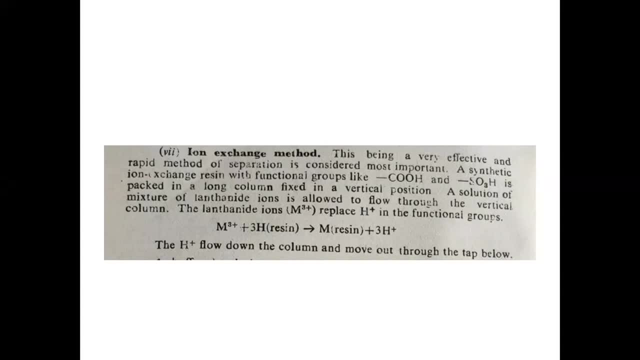 this. oh, what does it do? lanthanide and they come from the solution and travel down in the resin. resin come in the hand and resin which is h plus ion. this is h ion. this is replaced. okay. h ion is the resin maker. it does the work of replacing it, okay. 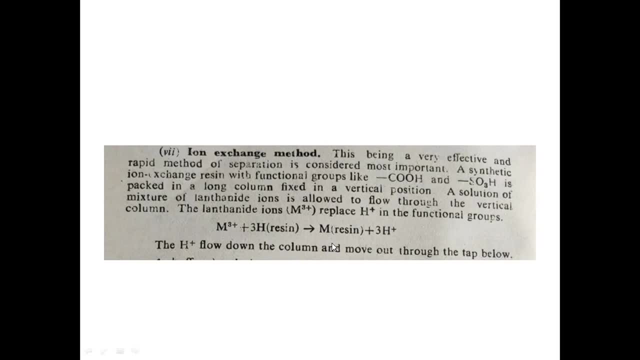 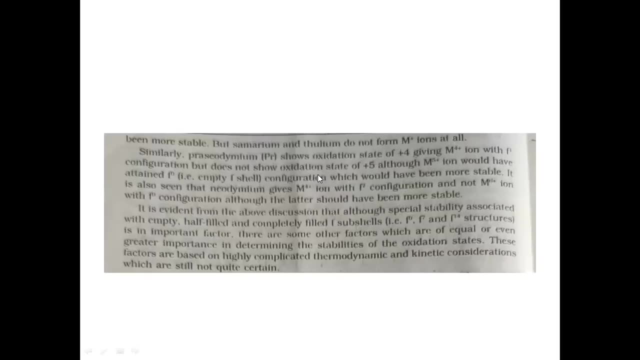 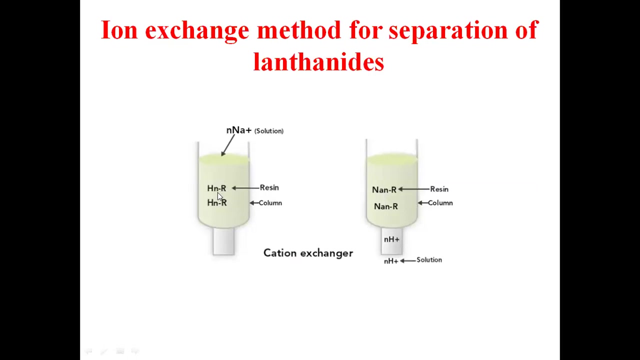 thus, resin will bind these m3 plus ions cations. they will bind to the resin. where is it now? It is in the resin. okay, it is in the resin. it is bound. okay, here the resin is being bind. you see, here the resin is being bind okay. 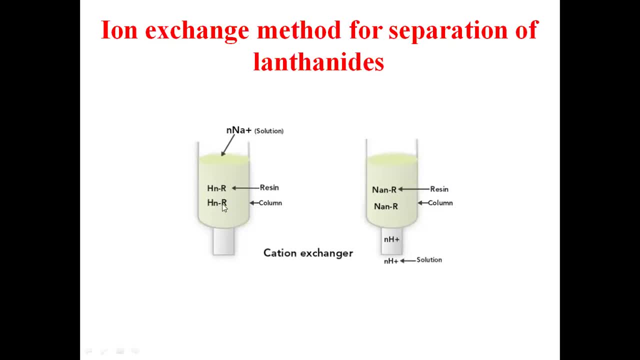 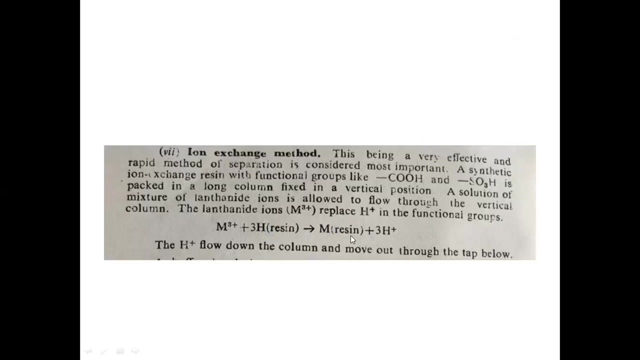 here the resin is being bind here. it is also there, okay, So what does it do? so what is it here? we have SO3 an here. we have put the solution here it is bind. now, what is left after binding from this? H plus, ok, it is bind here M resin. M means metal ion, lengthened ion, bind to resin. 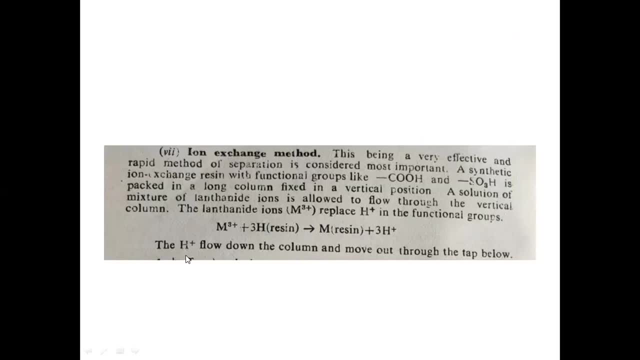 they are binded, they are attached to the resin. now, this H plus ion, they flows down the column and move out, out through the tap tap. we remove from the tap. then what is left? H plus ion is left, this H plus ion which we have replaced from the resin by means of this lengthened ion. lengthened. 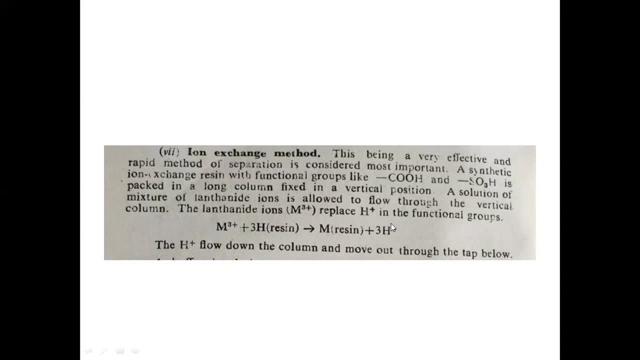 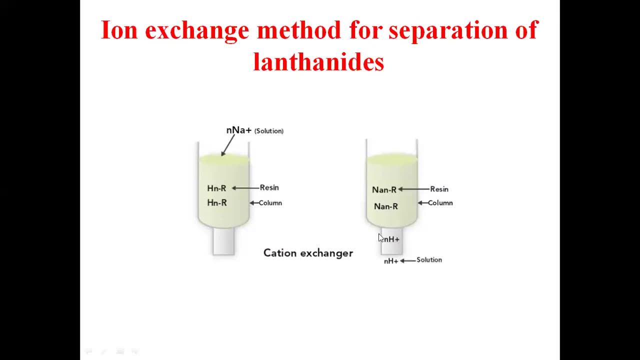 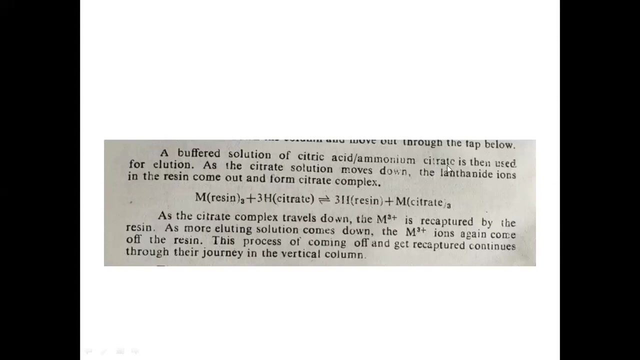 ion has replaced H plus ion, and this H plus ion is left. they will come out through the tap. it will come out from the inside of the tap. you can see here, replacement has been done. now buffered solution of citric acid and anion citrate is then used for elution. ok, now where is the lengthened ion? yes, 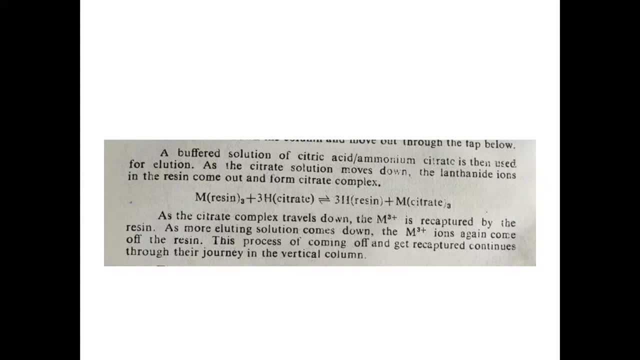 where is the lengthened ion resin? yes, they are binded to the resin. ok, they are bind to the resin. so now it is necessary to remove them from it, it is necessary to separate them from it. they are absorbed and attached to the resin, ok. so what we do to remove it? we use buffer solution. 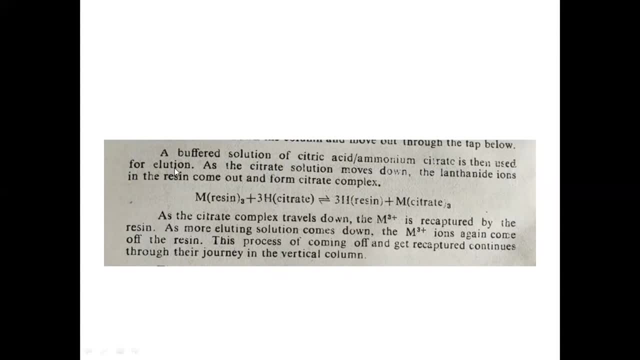 citric acid, citric acid and ammonium citrate. these buffers are used, use for illusion, to remove from them, to remove from the attached resin. it is also called illusion, or some books also call it leaching of the column: the column inside which has been fixed. it is gotta be separated from inside. 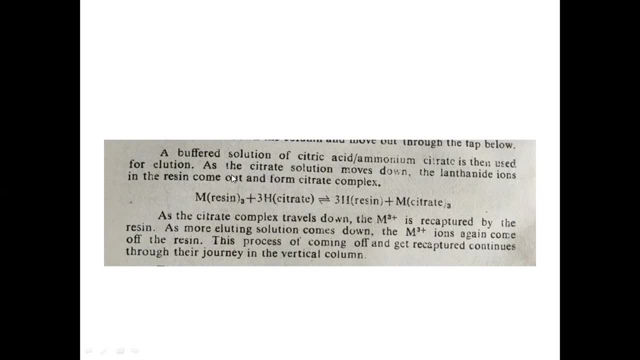 to separate this. we use buffer named as citric acid and amonium citrate. all right, what happens out of the box? we move the buffer from here and call for anonen citrate today, as we trash first buffer and let the buffer again affected by that buffer and scrunch it properly, then we move the buffer along with the buffer and then the buffer will come back to theomonium citrate. ok, 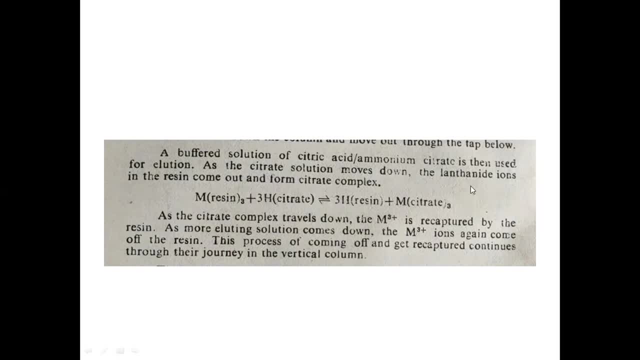 As the citrate solution moves down comes down, the lanthanid ions in the resin come out and they form the citrate complex. This is M-resin-3.. This is attached M-3 ion is our lanthanid ion, which is attached to the resin. 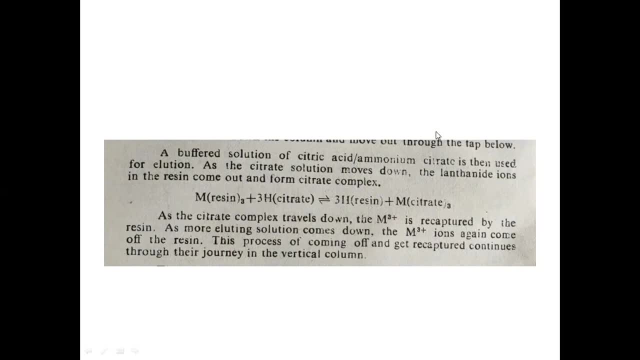 Now, what are we adding from above? We are adding citric acid, ammonium citrate solution, which is our buffer solution. Why are we adding? What is the role of that? What is the role of that buffer? Hello, what is the role of that buffer? 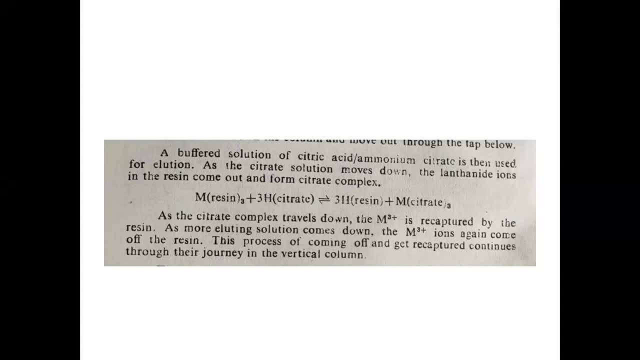 For elution: Yes, elution or leaching of the column. Elution: you have to remove from the column. We have to separate the lanthanid ions from the column. This is our buffer solution. We are adding buffer solution from above. 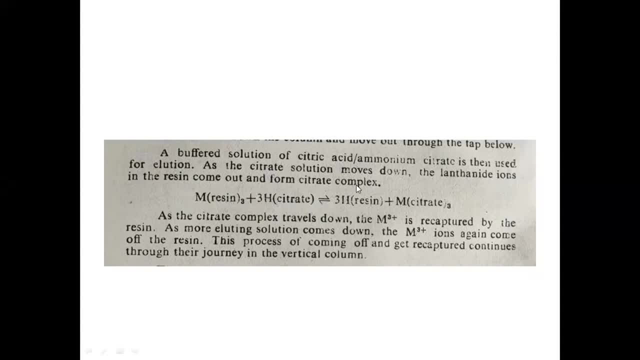 Lanthanid ions in the resin come out and they form the citrate complex. What are we doing? The citrate complex is formed. Can you see the citrate M-3 plus ion and citrate Citric acid? This is combined. 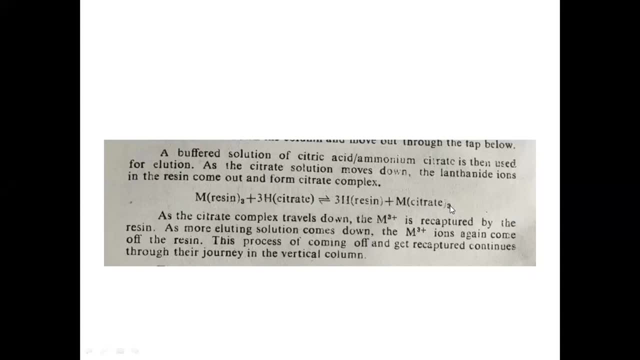 It is joined and attached. Citrate complex is formed like this: This resin is left, as it is 3H resin, Okay, As the citrate complex travels down. as the citrate complex comes down, M-3 ion is recaptured by the resin. 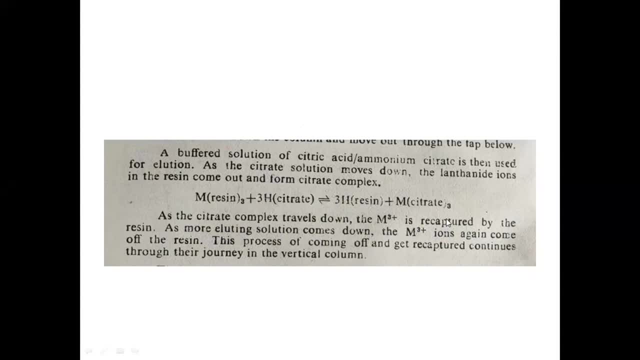 Okay, M-3 ion is our lanthanid ion. Then it is recaptured. How is it recaptured? From the resin? The resin recaptures it once. Okay, As more eluting solution comes down, M-3 ion again comes of the resin. 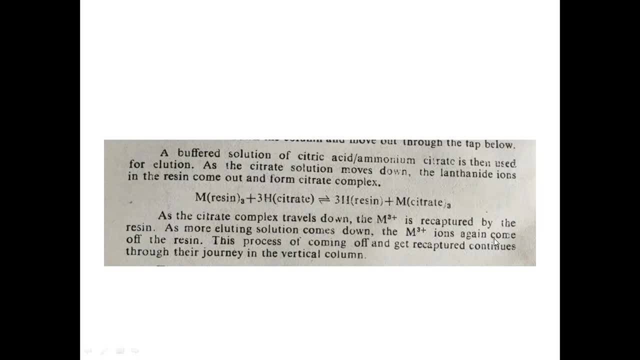 What will we do to remove it? Once again, we will add the eluting solution and this buffer solution. Okay, It has recaptured The resin, has removed the lanthanid ion which had come out. The elute was out After adding citric acid, after complex formation. what we have to do again is to add more eluting solution. 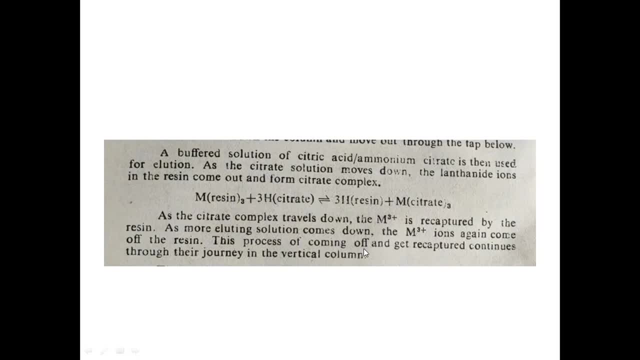 What is the eluting solution? We have to add citric acid and ammonium citrate. So what will happen? As more eluting solution comes down, M-3 ion again comes of the resin. Do you understand? It will come out again from the inside of the resin. 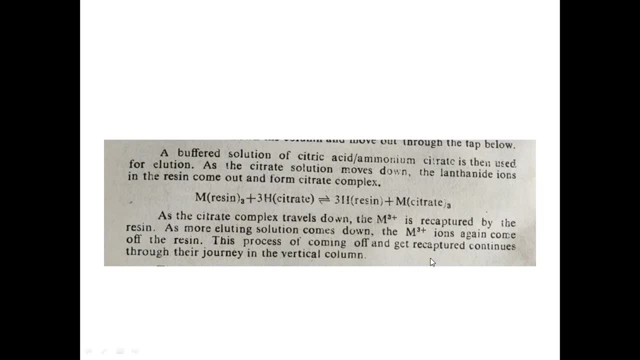 As we increase its quantity. once again, our citrate will come out. Once again, we will add citrate from the top of the buffer solution. What will happen after adding it? It will come out Okay. This process of coming off and getting recaptured continues throughout their journey in the vertical column. 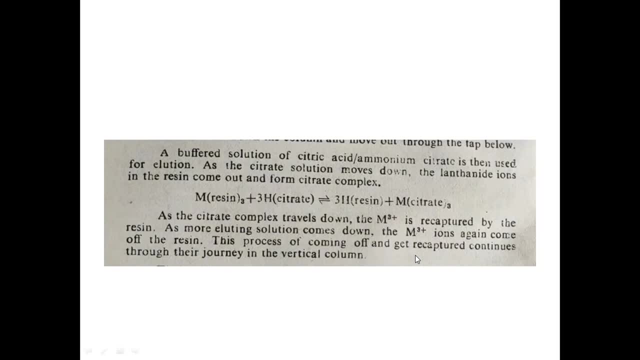 This process keeps repeating. Okay, To come out from it. we will add our complex. Okay, After adding the complex, it will recapture from it. It will get attached to the resin Once again. we will add a lot of citric acid, ammonium citrate solution and then it will come out in the glass. 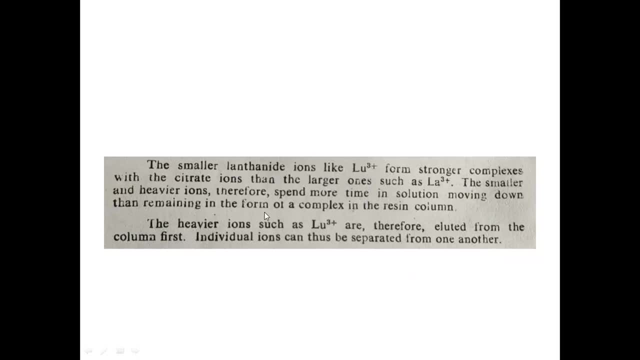 The smaller lanthanid ions, like Leutacium. they form stronger complexes with citrate ions. There are small ions in the lanthanide series. We are talking about small ion with lanthanid contraction. Okay, So when we go from lanthanum to lutetium, atomic size, ionic size- it goes on decreasing. 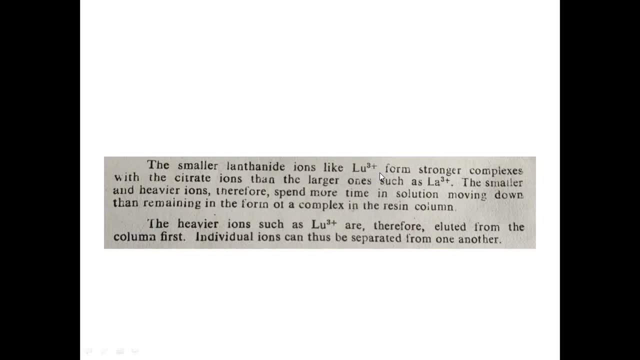 That is called as the lanthanate contraction. So lutetium 3 plus is the smallest size. So what does it do? It forms a stronger complex with citrate ions, Then larger ones. Where is lanthanum? We are taking lanthanum from the beginning. 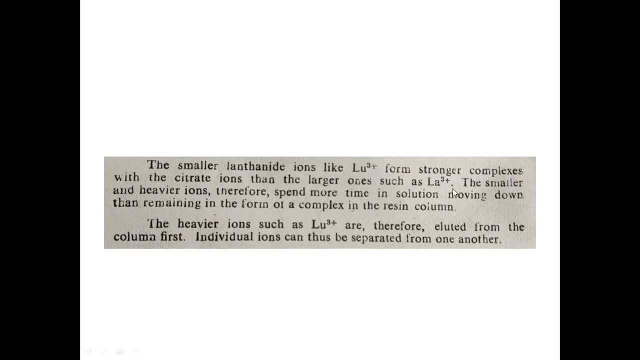 So when we are going from lanthanum to lutetium, the size gradually decreases. This is called as a lanthanate contraction. That is why lanthanum is in the largest size and lutetium is in the smallest size. 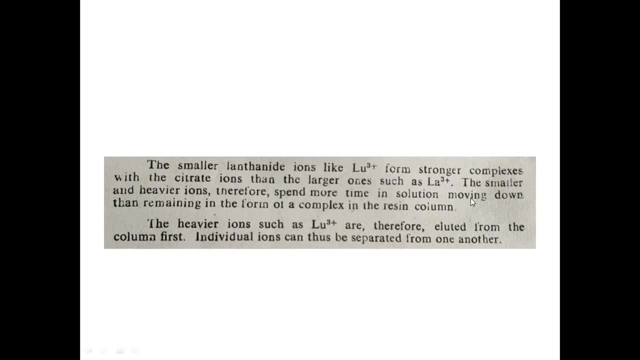 That is why it forms a stronger complex with citrate ions, The smaller and heavier ions, therefore, they spend more time in solution. So in solution they spend more time moving down, then remaining in the form of complex in the resin solution. 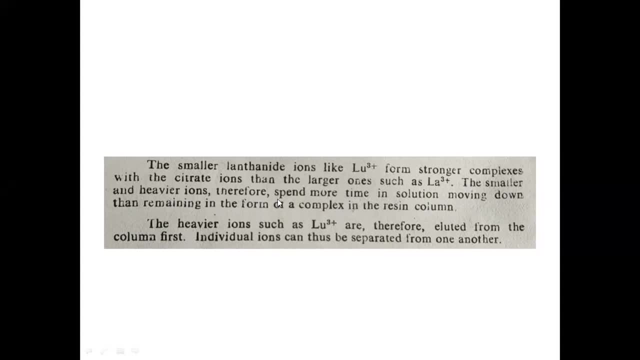 Okay, The smaller ions and heavier ions: Okay, So in solution. they spend more time in solution, moving down, then remaining in the form of complex in the resin column. Okay, So in solution. they spend more time in the smaller and heavier ions, such as lutetium 3 plus, are therefore eluted from the column first. 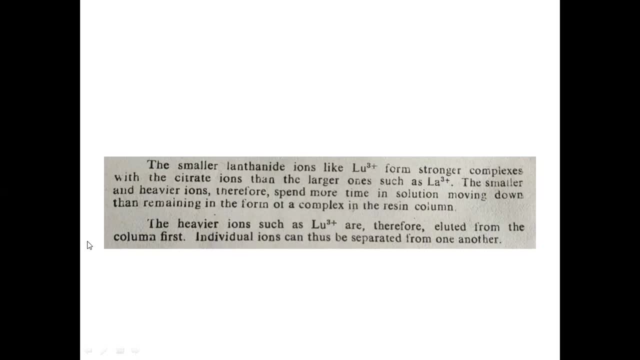 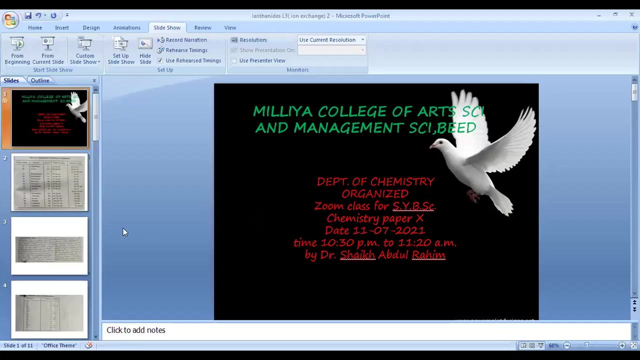 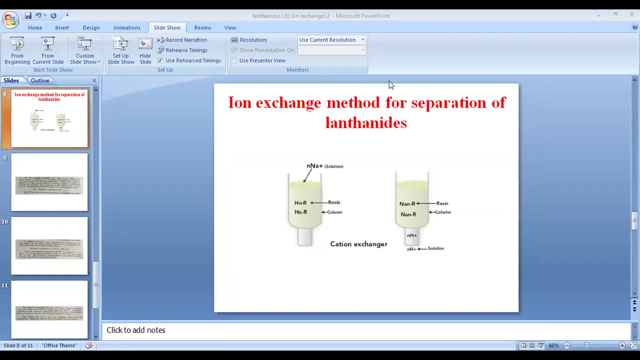 That is why, lutetium ions, they are suppressed, So they come out of the column first, Okay. And individual ions: we can separate them later from each other. Okay, We will cover only this much in today's material, Okay. 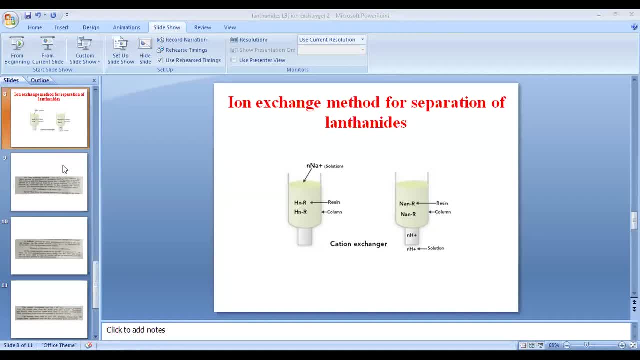 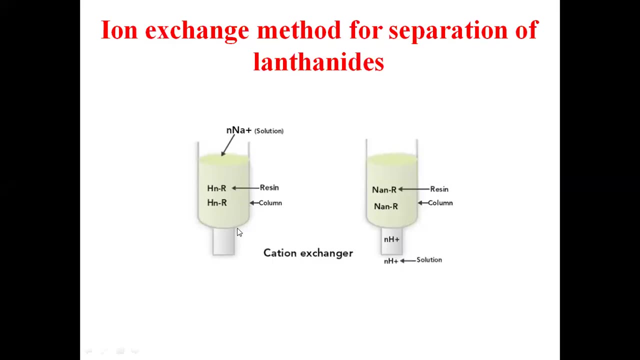 Ion exchange method. What are its principles? How does it operate? What is the process? Okay, This is our column. it has a murate, like a vertical column murate. it is filled with resin. It has synthetic resin. it has COH, SO3H, sulfonic acid and carboxylic acid ion. 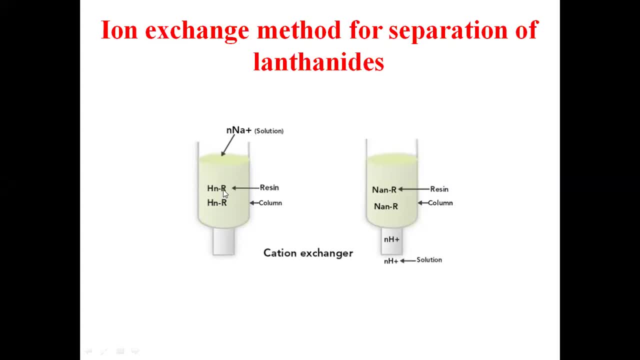 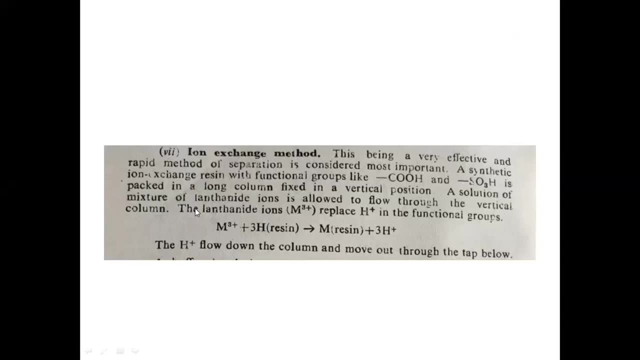 We add solution from above. lanthanidine is replaced, EH plus cyan is replaced and attached to the column. To elute it from the column, we add solution from above: citric acid, ammonium citrate. Here it is binding to the resin. after that what comes out of the tap is EH plus cyan. 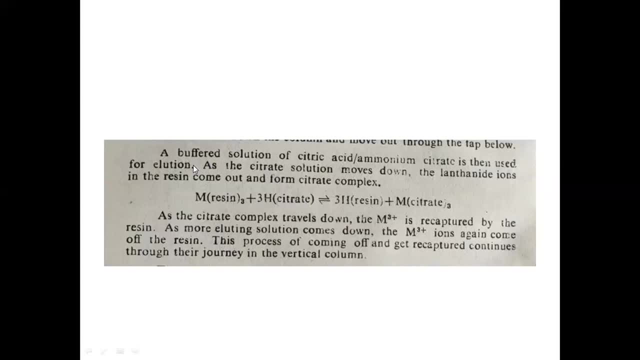 Then to remove the attachment, to elute it, to leach the column, we use buffer of citric acid and ammonium citrate. It forms a complex with EM3 plus lanthanidine. It comes down. the complex comes down a more elutinous solution and it is recaptured by double. 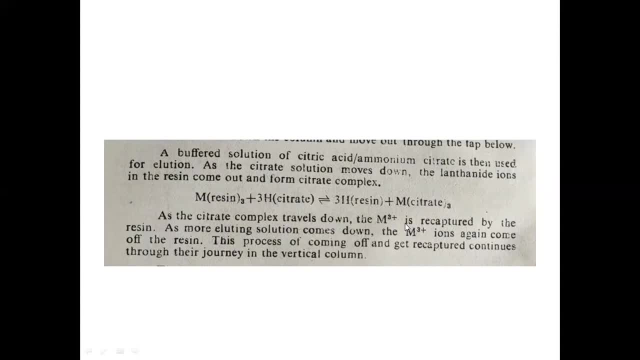 As the citrate complex travels down. As it comes down, the more elutinous solution and it is recaptured by double. So EM3 plus cyan and lanthanidine are recaptured by the resin. Now to remove it for elution once again, we add our buffer solution: citric acid, ammonium citrate. 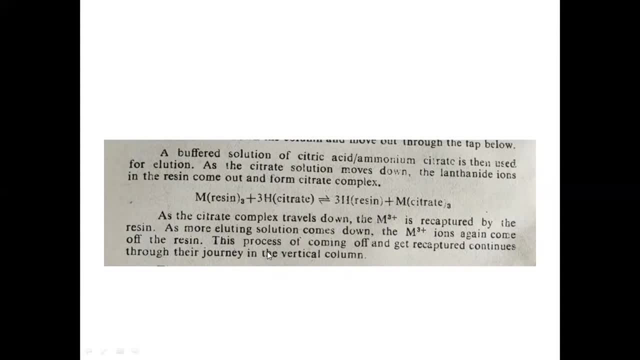 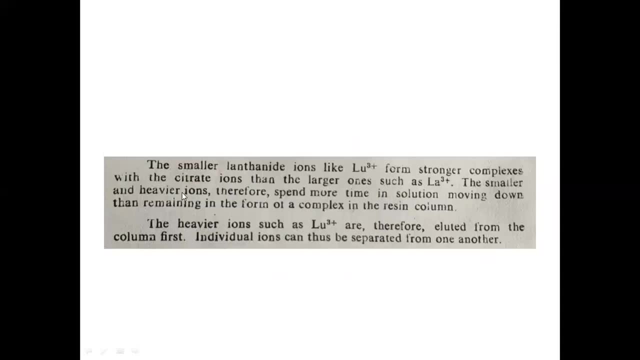 So EM3 ions again comes out of the resin. This process keeps repeating throughout the journey. The process repeats in the journey inside the column. The smaller lanthanidine ions. These ions form stronger complex with citrate ions as compared to larger ones. 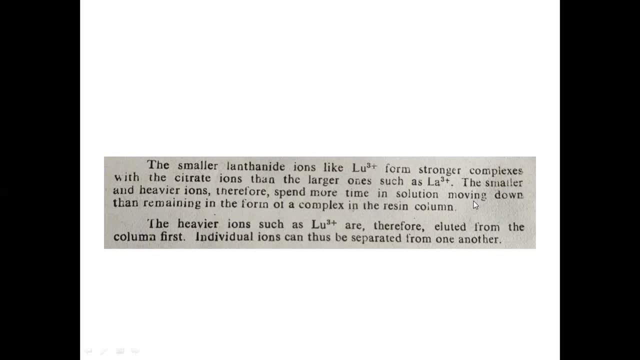 The smaller and heavier ions. therefore, they spend more time in solution, Moving down, then remaining in the form of complex. They remain less in the form of complex and spend more time in solution. So what happens? The heavier ions, like LU3 plus. they are therefore eluted from the column pass. 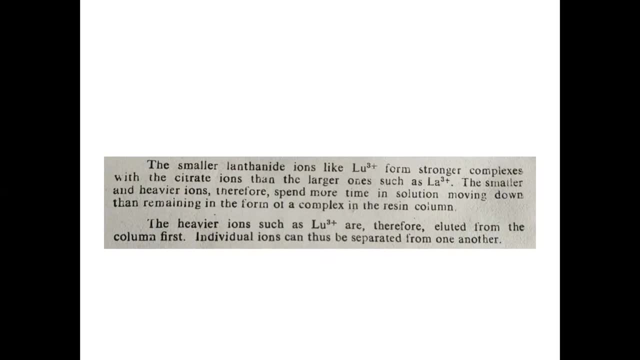 First of all, they come out of the column. After this we can separate the individual ions from the other processes. Okay, If you have any difficulty, you may ask. Whatever home assignment it is given through small questions. you should go for that.